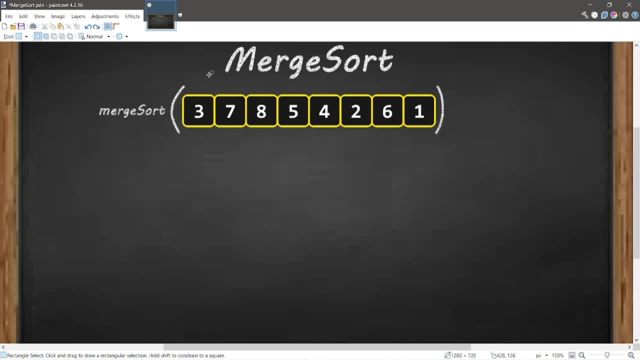 algorithm. Basically, what we do is that we will pass an array as an argument to a merge sort function. This function is going to divide our array in two. We have a left array and a right array. These will be subarrays, and we will copy the elements over from our original array to our 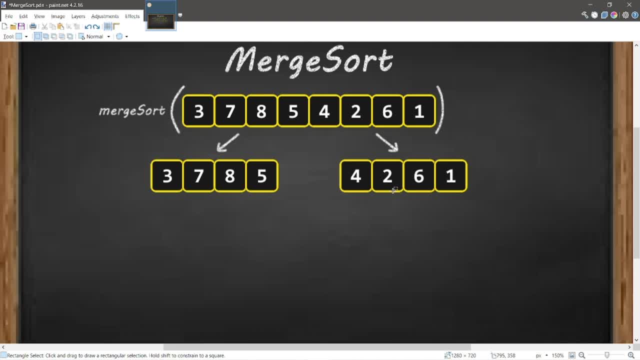 two new subarrays And merge sort is a recursive function, so at the end of merge sort we will call merge sort again and pass in our subarrays that we create. And again the merge sort function is going to divide our arrays in two by creating two new subarrays and then copy the elements over. 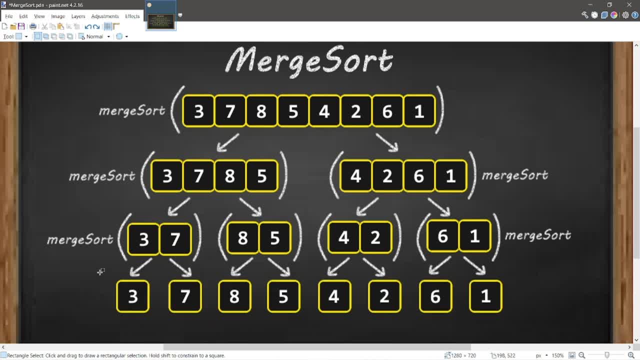 and we will stop when our arrays only have a size of one. And that's where sorting, then merging, come in. And with the process of merging and sorting we will create a second helper function named merge. Merge will accept a total of three arguments: our left subarray. our right subarray. 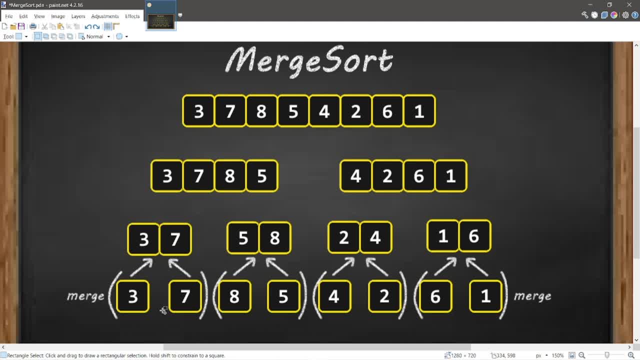 and the original subarray in which these elements came from. Merge is going to take these elements and put them back into their original array in which they came from in order, and we will do the same thing with the next grouping of arrays until all of these elements are merged back into. 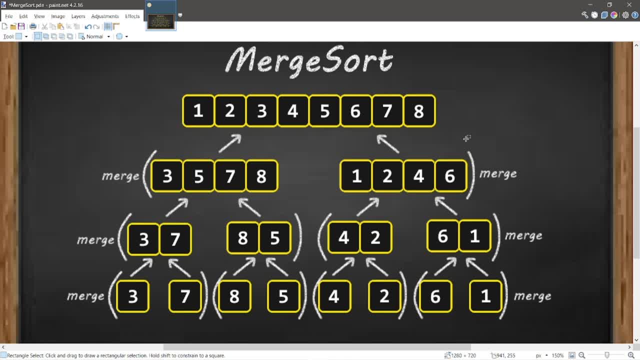 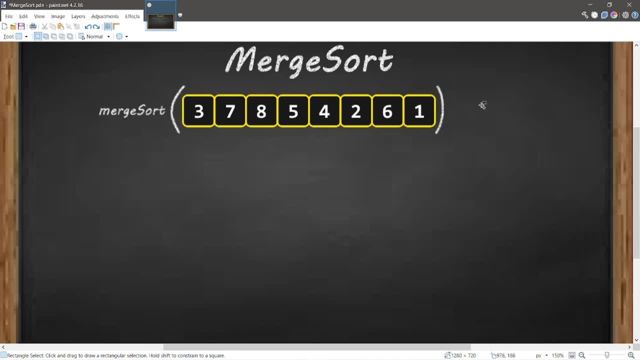 their original array in which they came from, And then we will do the same thing with our all in order. Now, in practice, when we do execute this merge sort function, instead of tackling all of these subarrays like one layer at a time, we will tackle them by one branch at a time. So it's 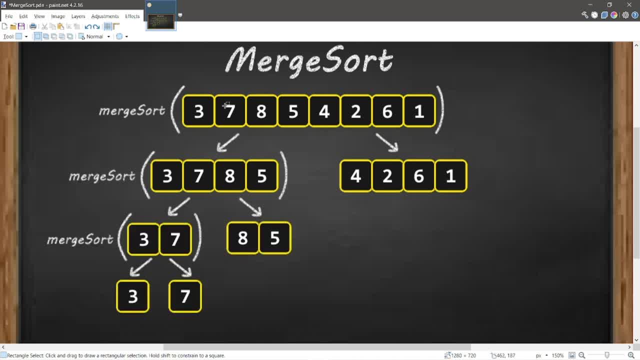 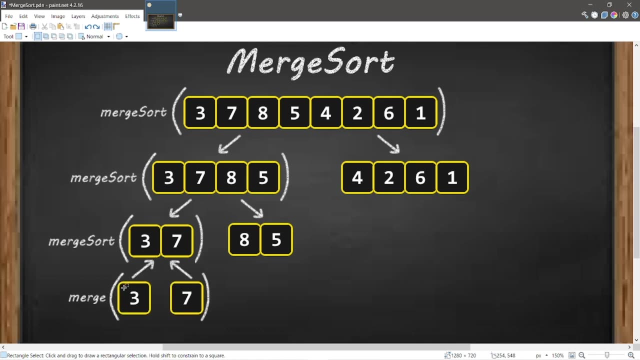 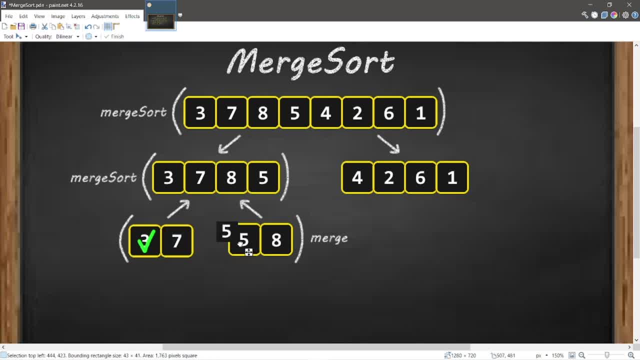 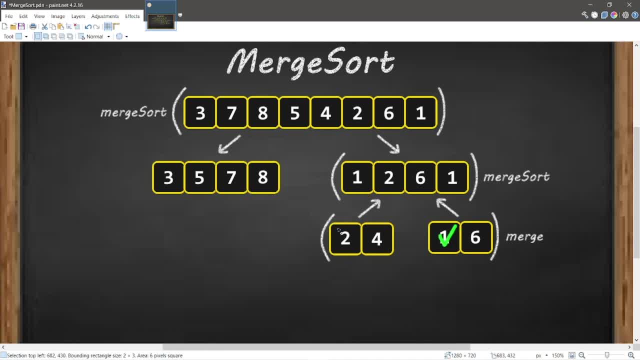 And what we do is we are going to take our array up for test-run And we are going to find the array And we then go back to demo training. So now, by using R phi, we're going to get a new array. 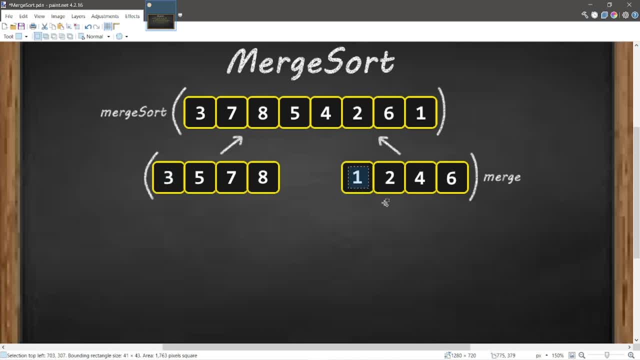 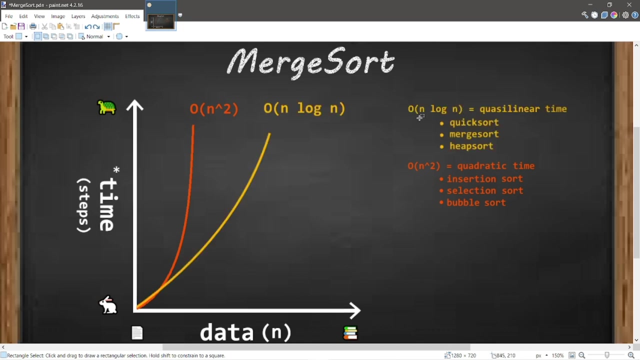 And, as I said, we're going to run a new set up And here we have our kilometer type array And I think that's all our learning icon, Thank you. Thank you, MergeSort is faster than InsertionSort, SelectionSort and BubbleSort. 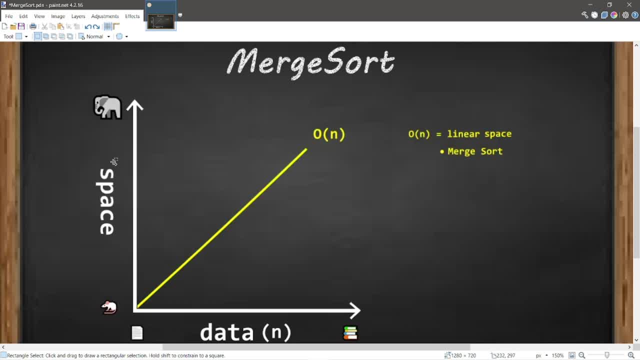 But on the other hand, the MergeSort algorithm uses more space than BubbleSort, SelectionSort and InsertionSort, because we need to create new subarrays to store elements, whereas BubbleSort, SelectionSort and InsertionSort can sort in place. 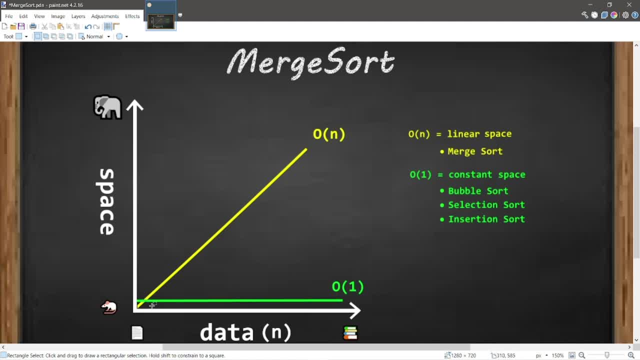 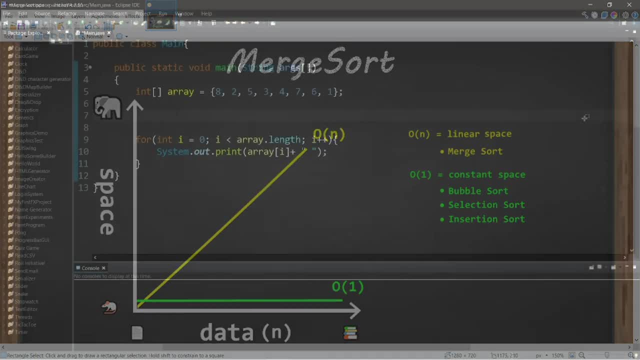 so they use a constant amount of space to do their sorting, unlike with MergeSort. Now let's move on to the hands-on portion of this video and create a MergeSort function in code. now All right. Well, let's get started. 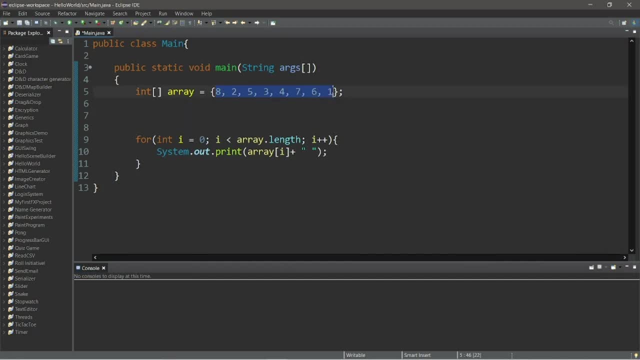 We'll need an array to work with, make up some numbers, make sure that they're not in order, as well as a for loop to iterate over the elements of our array. So currently our array is not in order, but that's going to change soon. 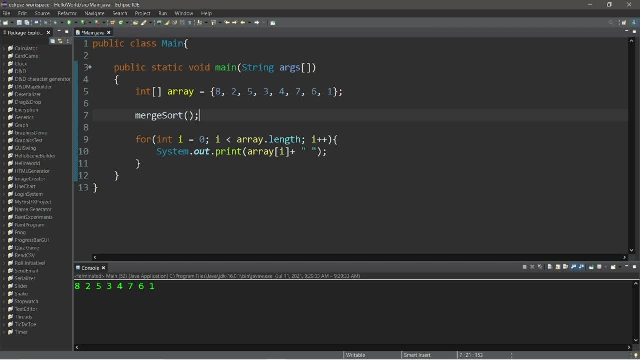 Let's invoke a MergeSort method that we still need to declare. This is going to be a recursive method and we will pass in an array, And each time that we invoke this method, we will split our array in half, create two subarrays and then copy the elements over. 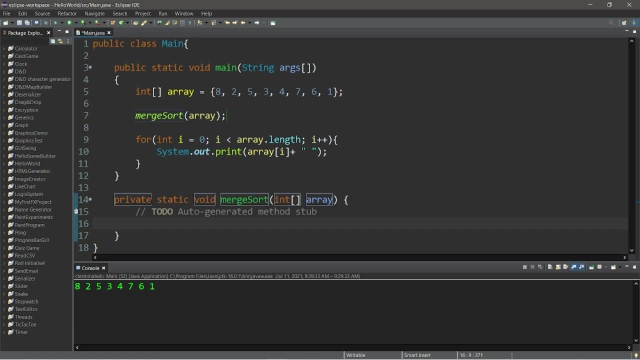 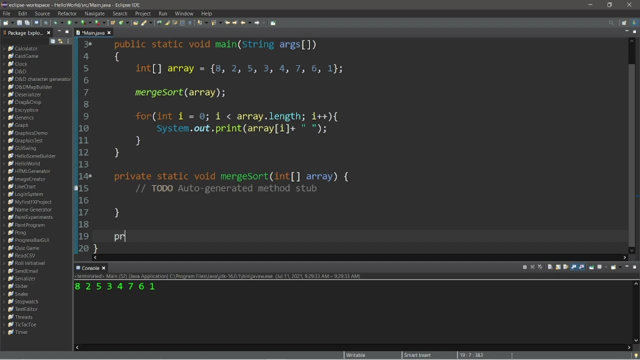 So let's create, We declare this method PrivateStaticVoidMergeSort, and we'll need a helper method too, and we'll name this Merge. A helper method is just a method that helps another method, basically So PrivateStaticVoidMerge. 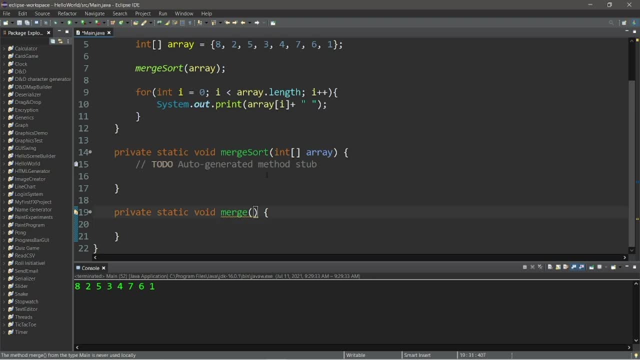 And there's going to be three parameters within our Merge method: Int LeftArray, Int RightArray and Int Array. Remember that these are arrays of integers. The first thing that we're going to do within our MergeSort method is that we need to get the length of our array. 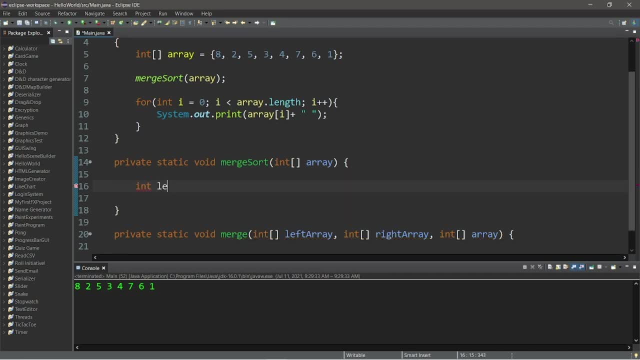 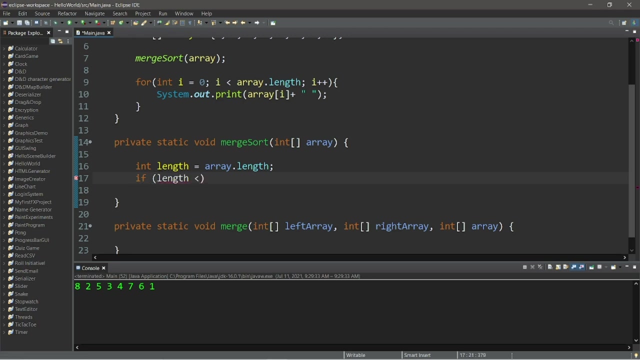 So let's cache that within a local variable named length. Intlength equals arraylength, And we'll need a base case too. When do we stop recursion? If length is less than or equal to 1,, then we should, And this is our base case. 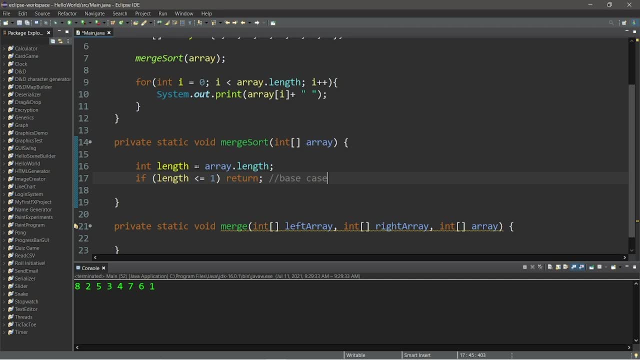 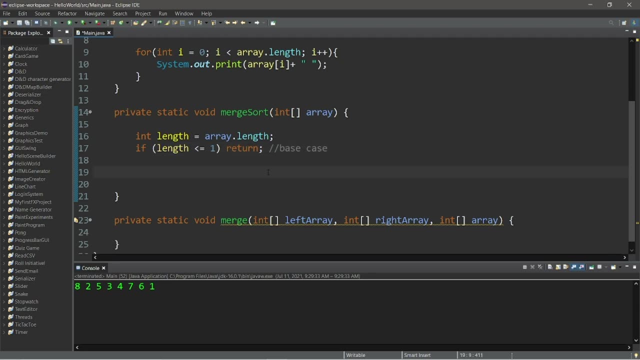 Basically, with this MergeSort method, we're dividing our array in two each time. If the length is 1, there's no longer a need to divide our array further And we'll need to find the middle position of our array. Intmiddle equals length divided by 2.. 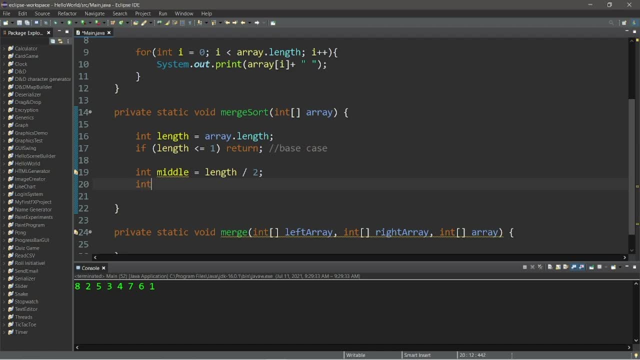 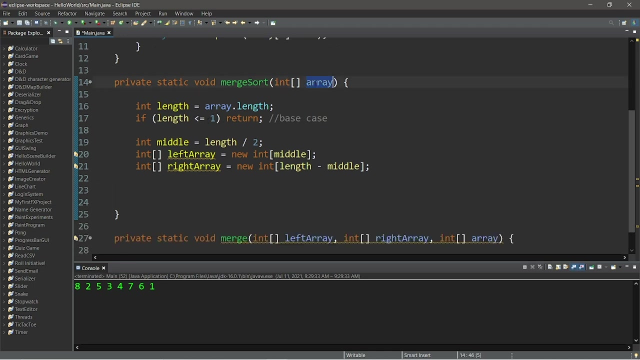 And we'll create two new subarrays. IntarrayleftArray equals new Intarray and the size is middle, And we'll create a right array: IntarrayrightArray. The size is length minus middle. Okay, now we need to copy the elements of our original array to our left and right arrays. 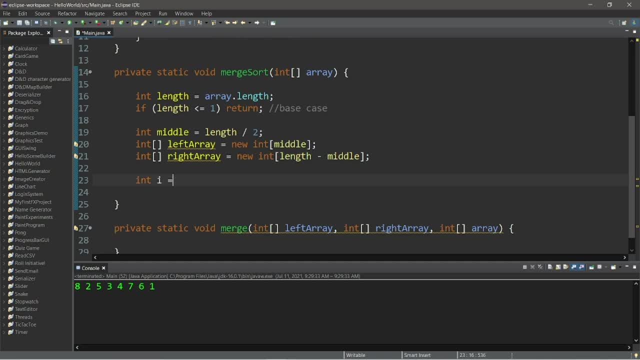 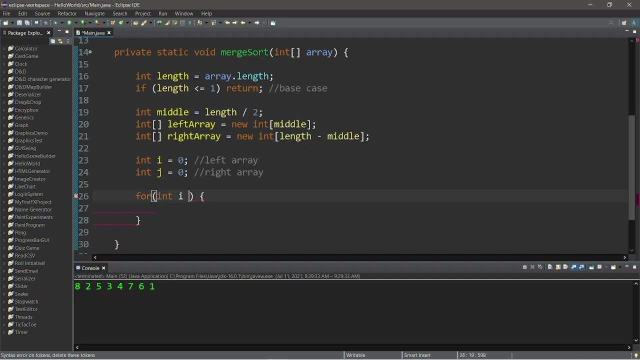 So we'll need two indices: Inti equals 0. This will be for our left array, And Intj equals 0. And this is for our right array. Then let's create a for loop. We don't necessarily need to declare a new index here. 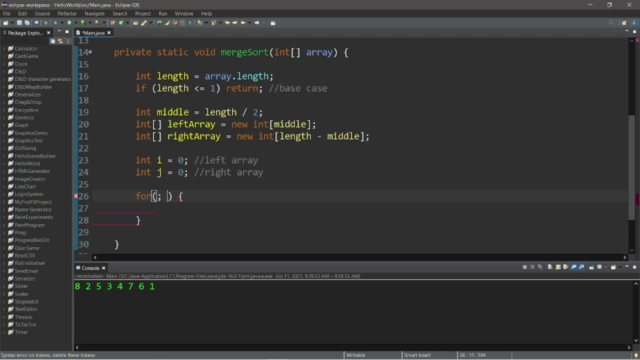 We can just use i, So I'm going to add a semicolon. Our condition is: i is less than length, Then increment i by 1 during each iteration. So our condition is with an if statement if i is less than middle. 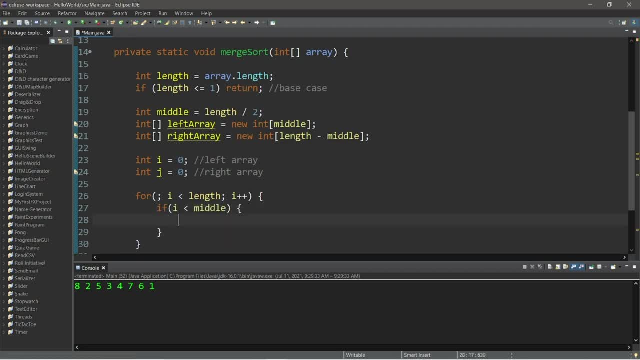 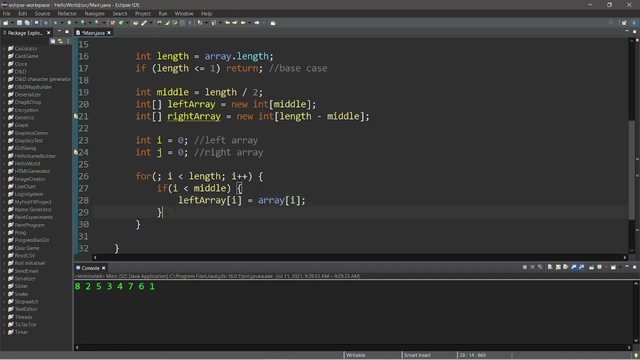 then we will copy an element from our original array to our left array, leftArray at index of i- equals array at index of i- Else we will copy that element to our right array, Else, rightArray at index of j. Remember that this index is for the right array. 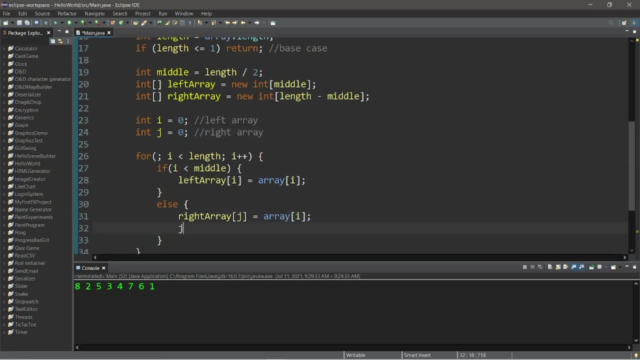 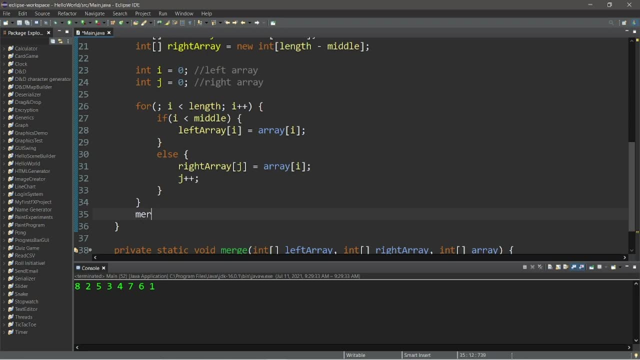 equals array at index of i. Then let's increment j by 1.. Okay, this is where recursion comes in. So outside of this for loop, we will call mergeSort again And pass in our left array. So we'll consistently divide our array in half. 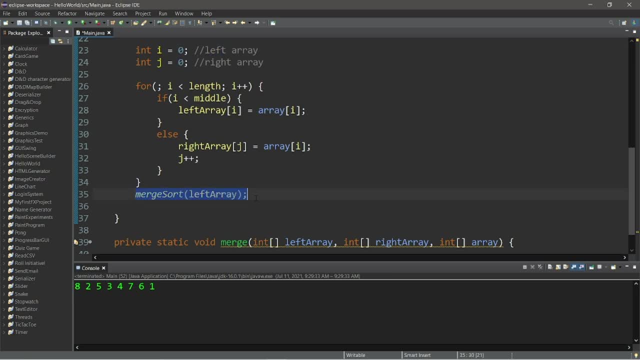 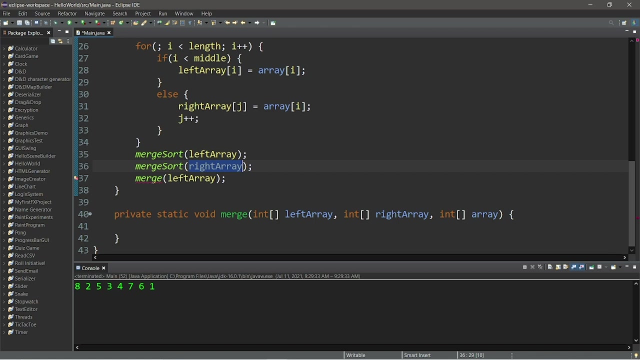 We'll begin by dividing the left array, then the right array with a separate recursive call, so left array, then right array and then call merge. So with merge we have to pass in our left array, right array and our original array, because we'll put the elements back in order. Left array. 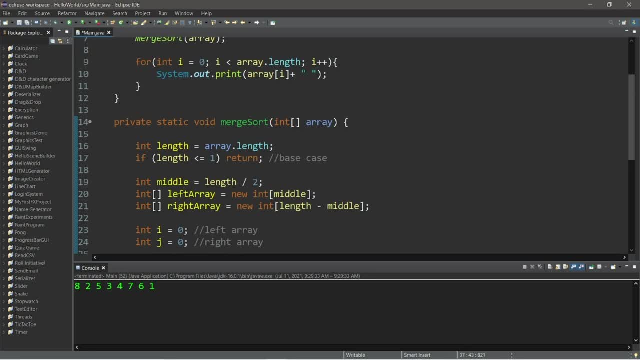 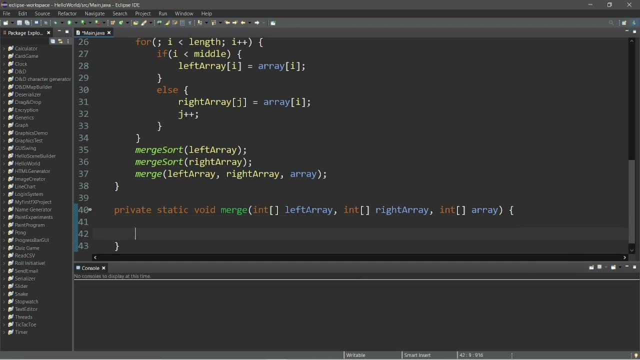 right array and our original array that we received as an argument. So that is it for the merge sort function. Let's work on emerge next. First thing that we're going to do within the merge method is cache the size of our left array and right array within some local variables. 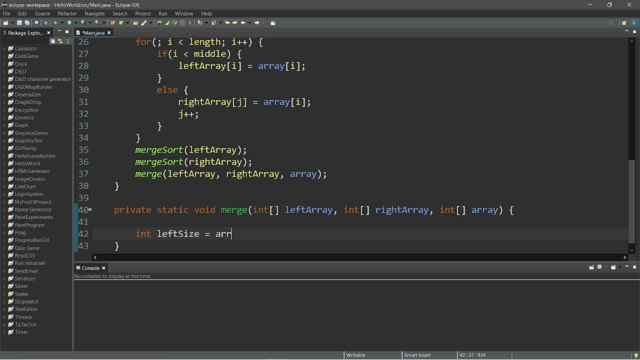 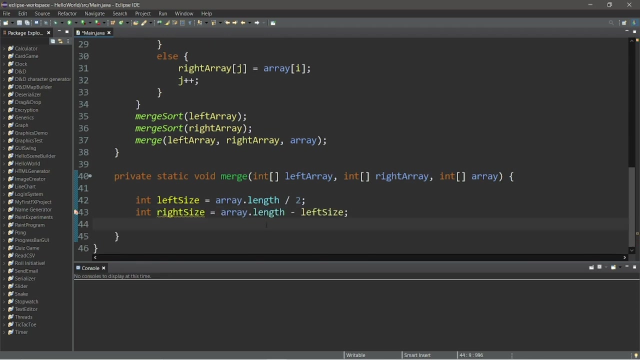 int left size equals array dot length divided by two. int right size equals array dot length minus left size. And then we'll need three indices: int i equals zero. This is for our original array to keep track of the position. L will be in charge of our left array and R? 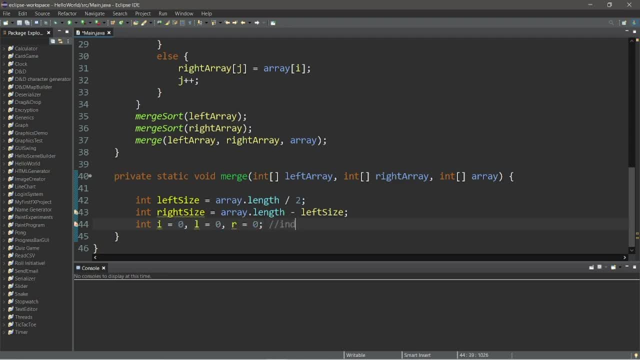 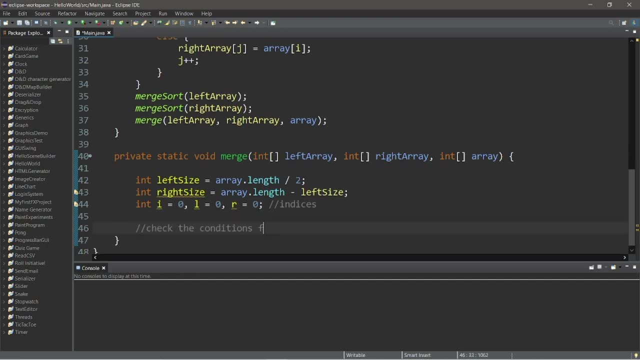 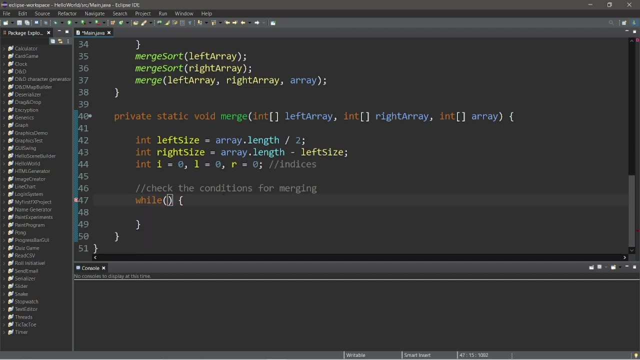 will be in charge of our right array And these will be the indices that we're using. Okay, the next part. we're going to check the conditions for merging, And we can do this with a while loop. So our condition is going to be: while l is less than left size and r is less, 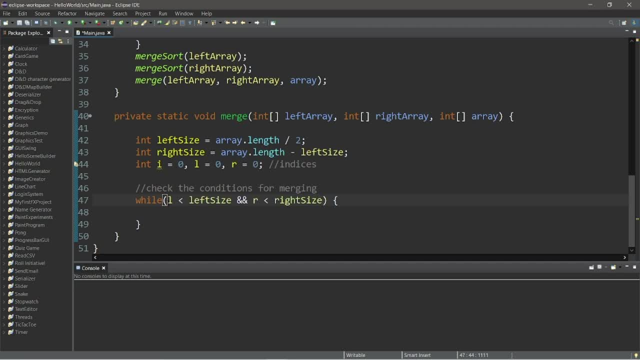 than right size. So, basically, while there's elements within both our left array and right array, we will continue adding elements to our original array And we'll need to check to see which element is smaller If left array at index of l is less than right array at index of r. 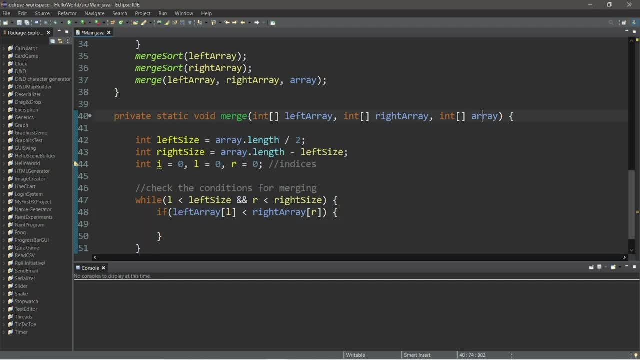 then we will copy the element from our left array to our original array. So we're basically comparing the number on the left to the right and adding whatever number is smaller back to our original array. So array at index of i equals left array at index of l. then we can increment I, increment l. 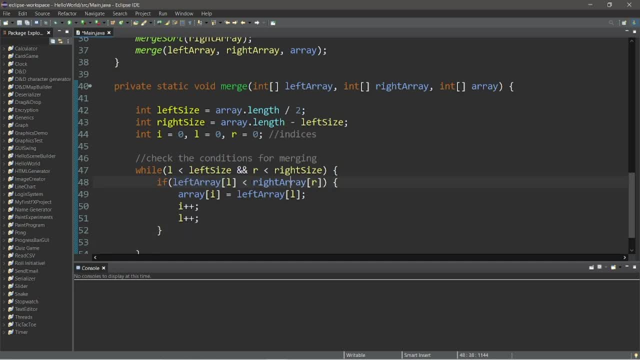 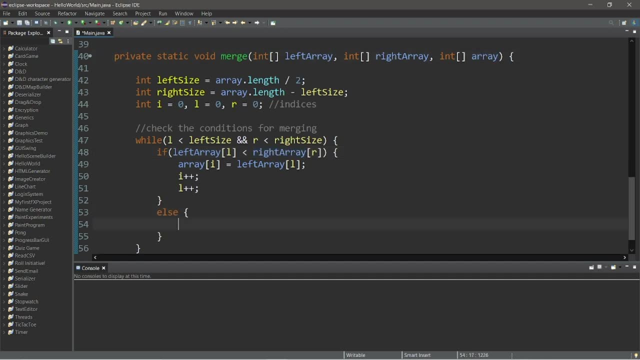 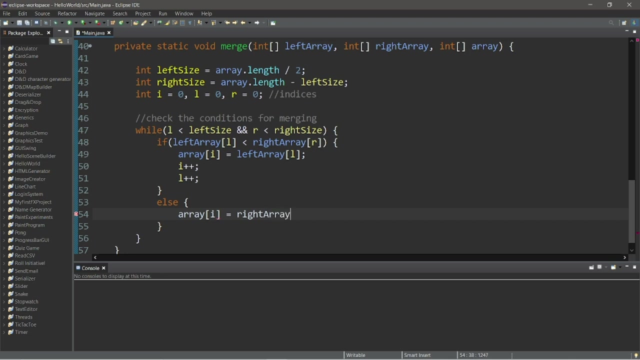 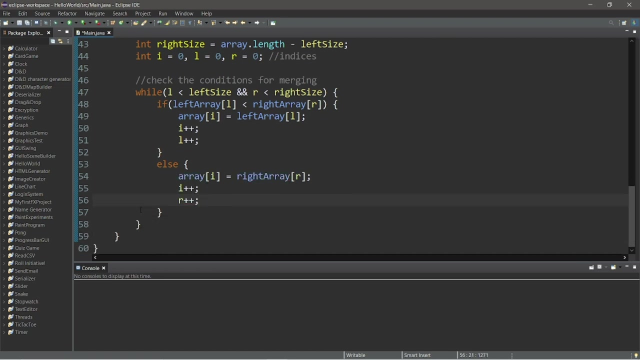 So if the number on the left is not smaller than the number on the right, we have to copy the L element in our right array to our original array and we can use an else statement: Else array at index of i equals right array at index of r. Increment i increment r. So there's probably 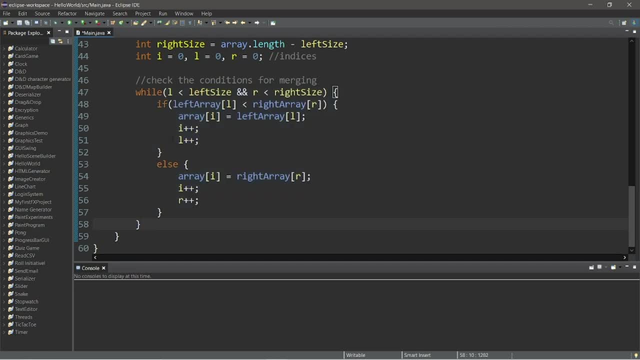 going to be one element remaining that we cannot compare to another element because there's only one left. So let's write a while loop for that condition. While l is less than left size, then we will take array at index of i equals left array at index of l Increment i increment l. 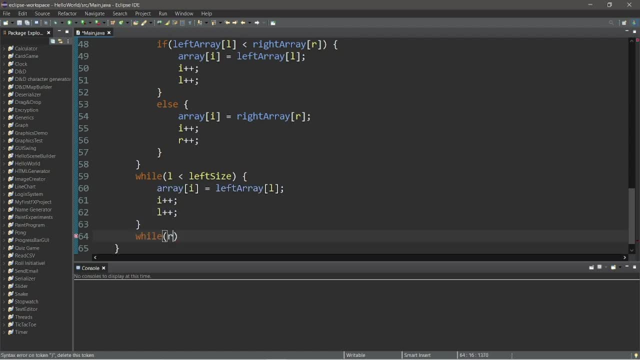 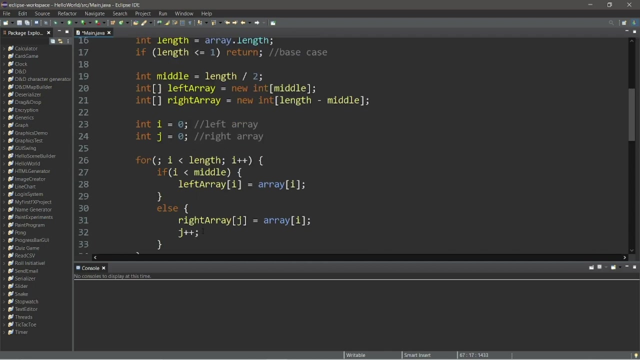 Then we'll need another while loop. If r is less than left size, then we'll need another while loop. If r is less than right size, we will copy the last right element over Array at index of: i equals right array at index of r. Increment: i increment r And that should be it. Let's run this: